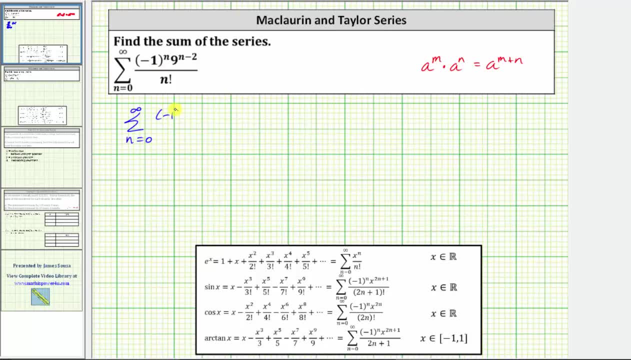 from n equals zero to infinity of negative. one raised to the power of n and then times nine raised to the power of n. times nine raised to the power of negative two, all over n, factorial. Again, notice how this product does give us nine raised to the power of n, minus two. 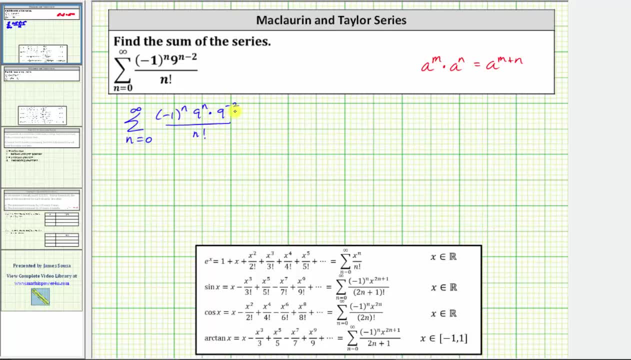 From here, nine raised to the power of negative two is not affected by n, which means we can factor this out and write this as: nine raised to the power of negative two times the sum from n equals zero to infinity of negative one raised to the power of n. 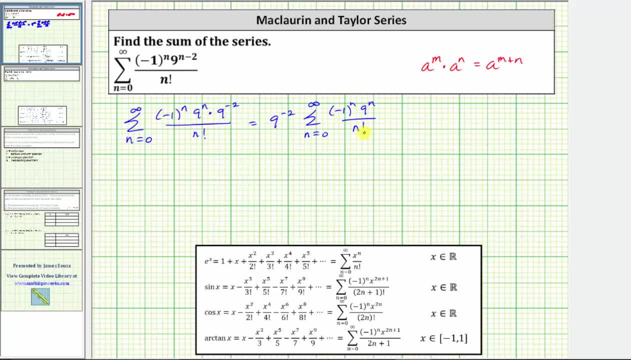 times nine, raised to the power of n all over n factorial. And now notice how the power on negative one and the power on nine are both n, which means we can now combine these by multiplying the two bases: Negative one, raised to the power of n. 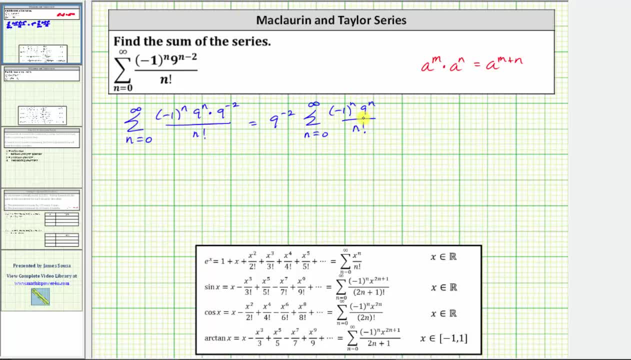 times nine raised to the power of n is equal to negative nine raised to the power of n, which gives us nine raised to the power of negative. two times the sum from n equals zero to infinity of negative. nine raised to the power of n, all over n. factorial. 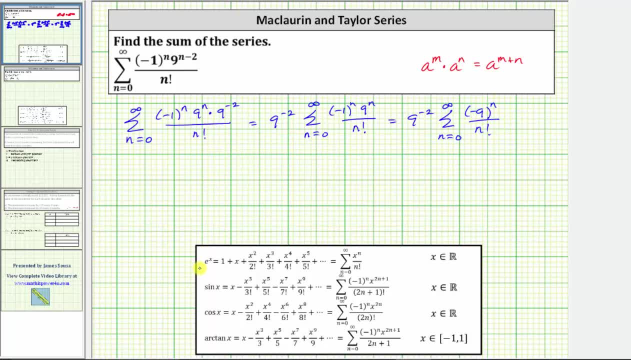 And now, if we compare this series to the power series for e to the x, it matches perfectly. Or x is equal to negative nine, which means this series is equal to e raised to the power of negative nine and therefore this product gives us the sum. 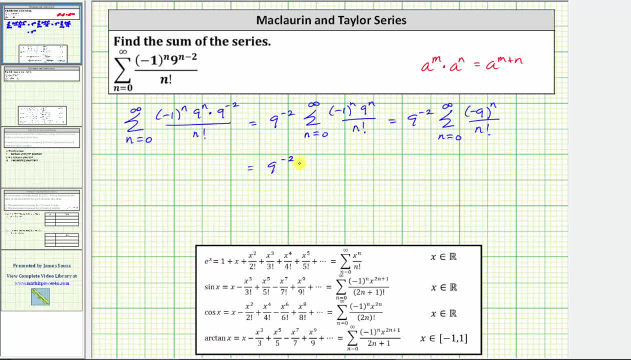 of the given series, which is nine raised to the power of negative, two times e raised to the power of negative nine. Let's rewrite this using positive exponents. This is equal to one over nine, squared e to the ninth. or, if we want, one over 81 e to the ninth. 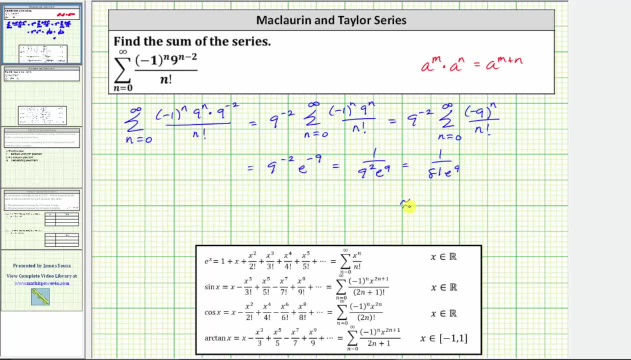 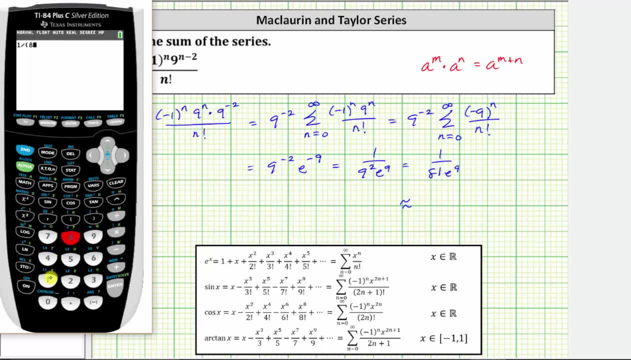 But let's also get a decimal approximation for this value. To do this we will use a calculator. We enter one divided by open parenthesis. 81 second natural log brings up e raised to the power of nine. right arrow, close parenthesis and enter. 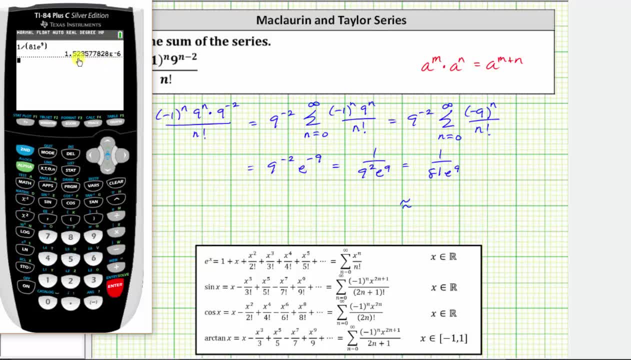 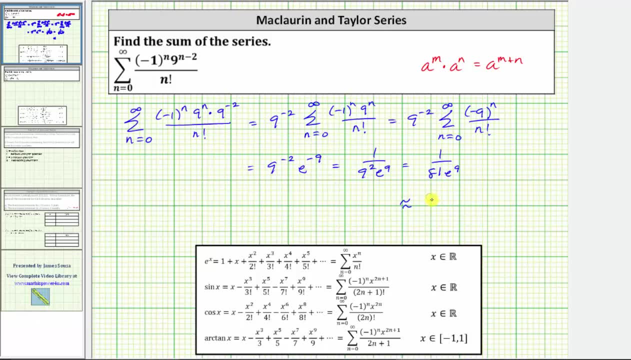 Notice how this is giving us scientific notation. Let's round this to 1.5236 times 10 to the power of negative six. That's one over nine, squared e to the ninth. That's one over nine, squared e to the ninth.